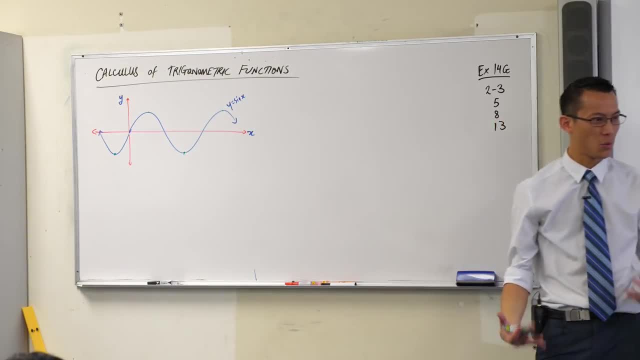 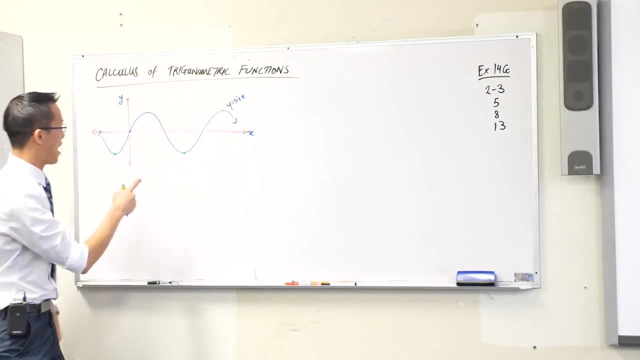 you should know exactly what the gradient is at those points. What's it going to be equal to? It should be 0, because what kinds of points are those? They are stationary points, right? Ah, local max, local min, etc. So at those points on this same graph, I'm going to put that's a 0 there for the gradient. that's what my other color's going to be. 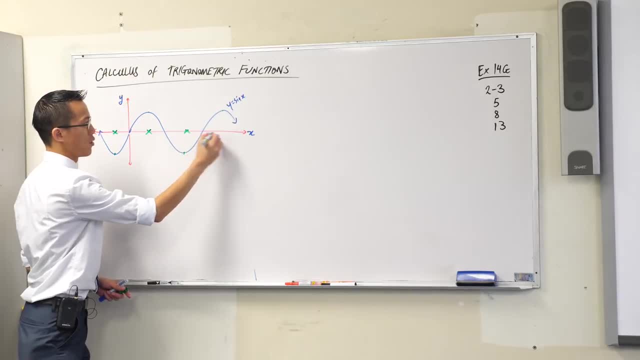 Here's another spot where the gradient is 0, and so on. Okay, Now I'm going to go one step further. Um, I just did a very rough graph. I didn't put any values on there. Okay, Now I'm going to go one step further. I just did a very rough graph. I didn't put any values on there. 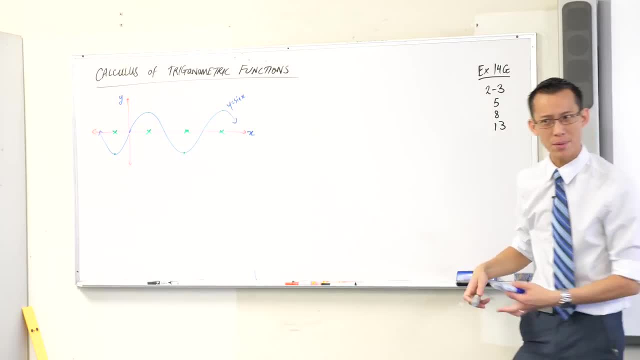 Okay, Now I'm going to go one step further. I didn't put any values on there. Okay, Now I'm going to go one step further. I didn't put any values on there, But you actually know those values right, Because we've been dealing with the sine curve for a while now. 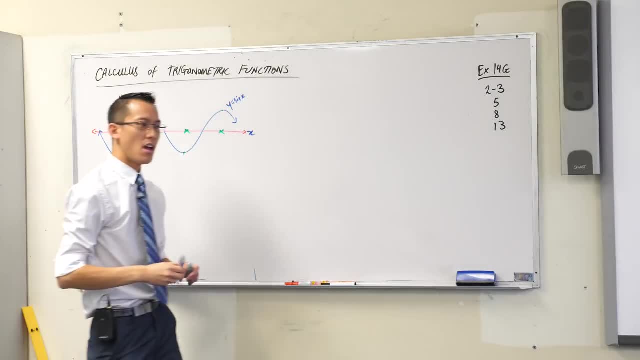 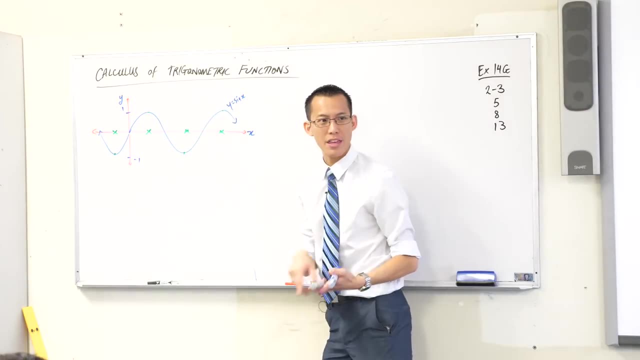 We know what its amplitude is, But in radians- and I'm going to come back to why it's radians in a minute- in radians, I wonder if you know those spots well enough to know their values. What's, um, this first stationary point? what's its value? 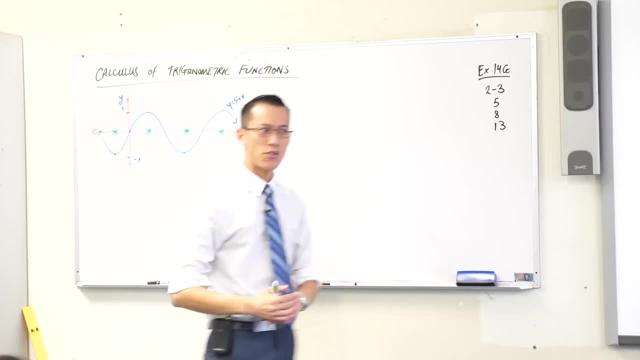 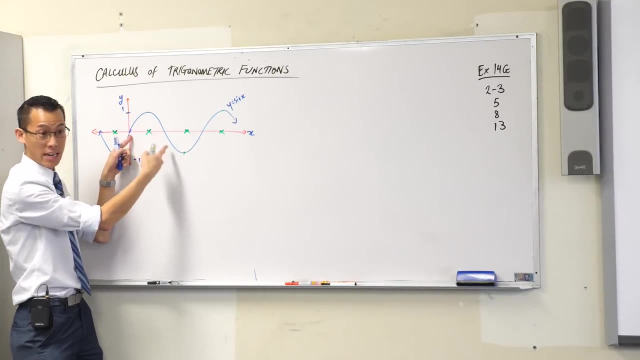 It's x value, It should be pi on 2, right, 90 degrees, Because if you think about it, here's 0 to 360, yeah, Oh sorry, there's 360.. So that's a quarter of the way there. So that's 90 degrees, that's pi on 2.. 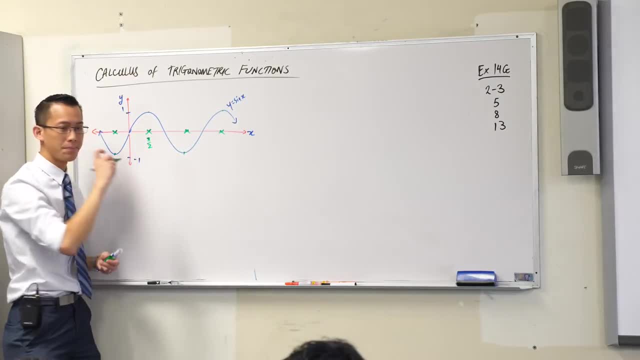 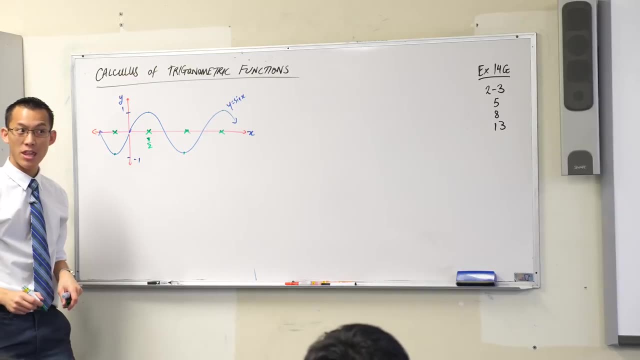 Let's write that in Pi on 2.. Your next one over what's that stationary point? That should be 3 pi on 2, right? Because look, it's 1,, 2,, 3 of them. So I'm going to write 3 pi on 2.. 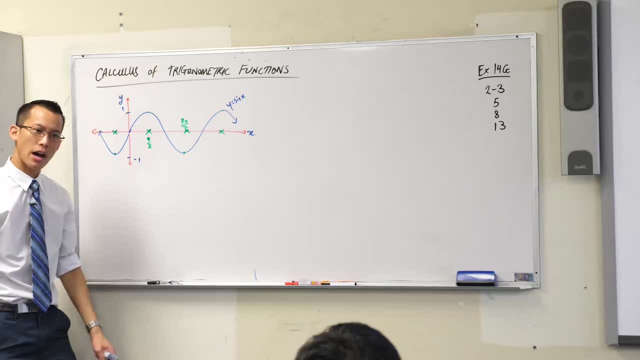 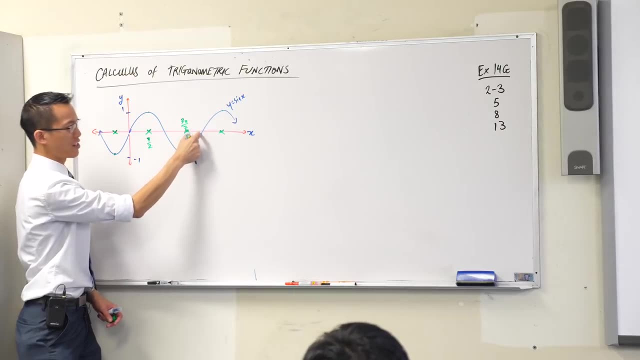 These ones out here are not in the normal domain in which I draw, but I think we can work them out right, Because, for example, this next one is: there's 3 pi on 2, I got another pi on 2 and another pi on 2,. 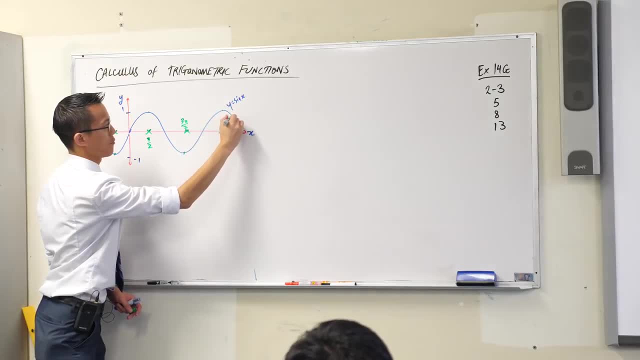 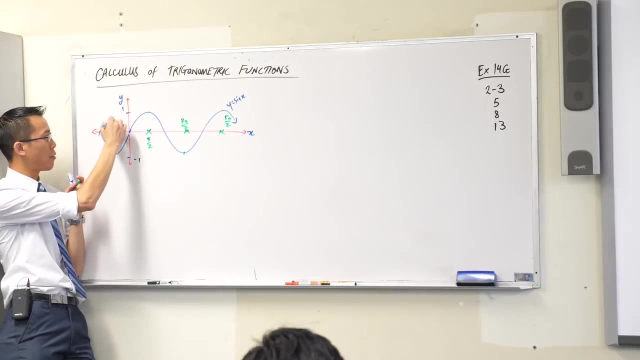 so it should be 5 pi on 2.. And what about this one back here? We don't usually draw this part. Yeah, it's just. you can see the symmetry of it, can't you? So I'm going to put negative pi on 2 over there. 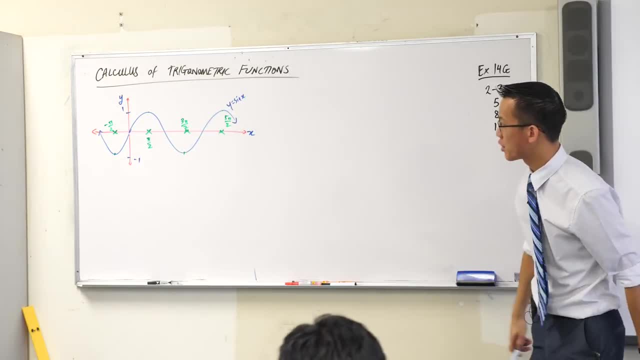 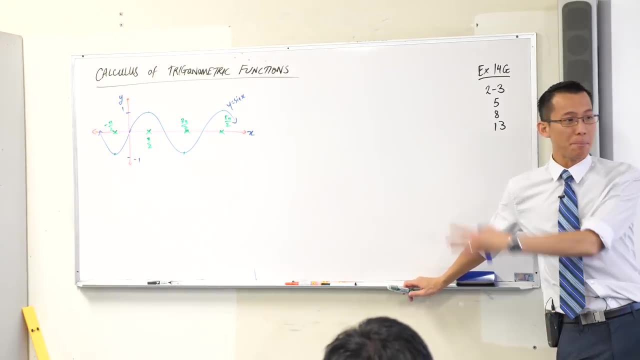 Okay, so far, so good. So I know a bunch of spots where the gradient is 0. But I can go more than that, right? Do you notice in between those stationary points, some parts of sine are increasing and some parts are decreasing. 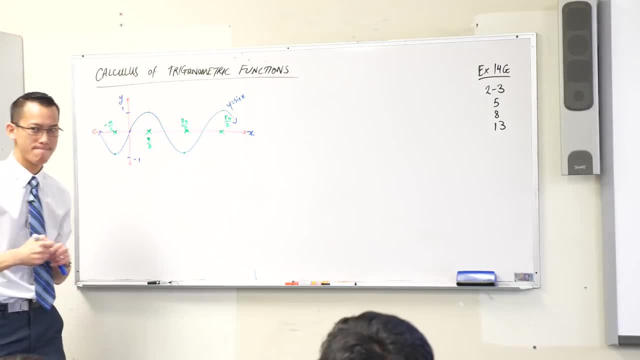 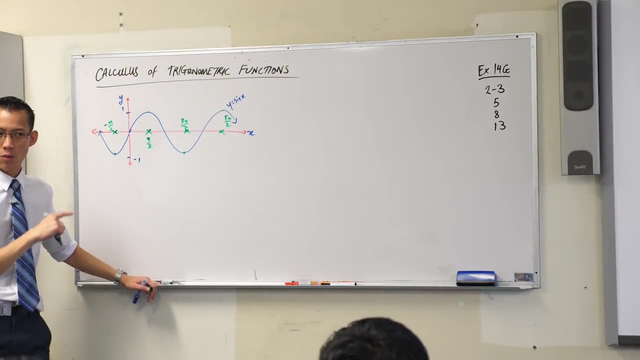 So when a function is increasing, what does that tell you about its gradient? It's going to be positive. It's going to be above the x-axis right. So where's the spot that you can see where you have an increasing function? 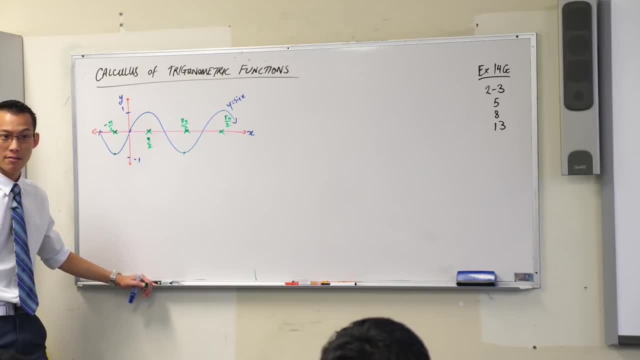 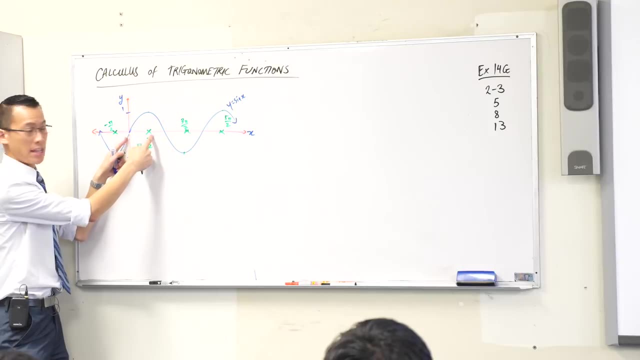 There's a whole bunch. Pick one Between 0 to pi on 2?. That's increasing. I think you could make it even bigger than that, couldn't you Like? I can see that this section here is also increasing. Do you get that? 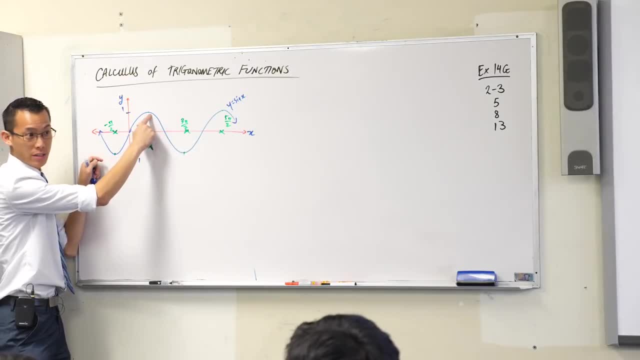 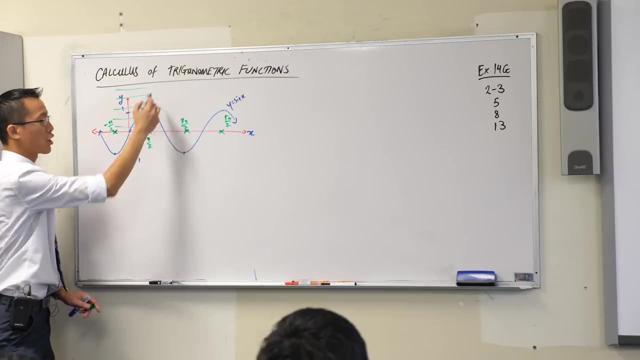 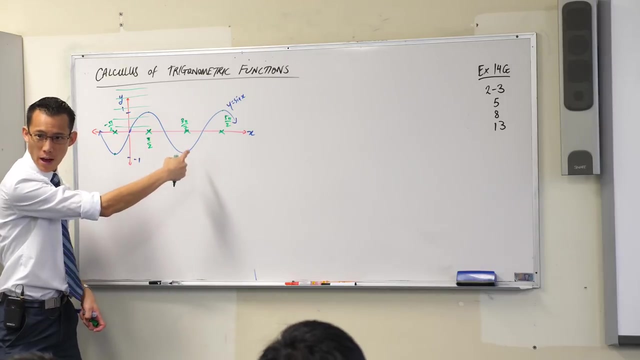 From here all the way up to here, it's increasing. So with this colour, which is my gradient colour, I'm going to show that up here the gradient should be positive. By the same logic, but in reverse, having a look between pi on 2 and 3, pi on 2,. 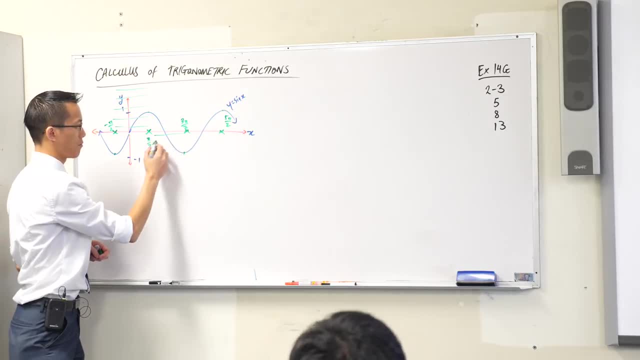 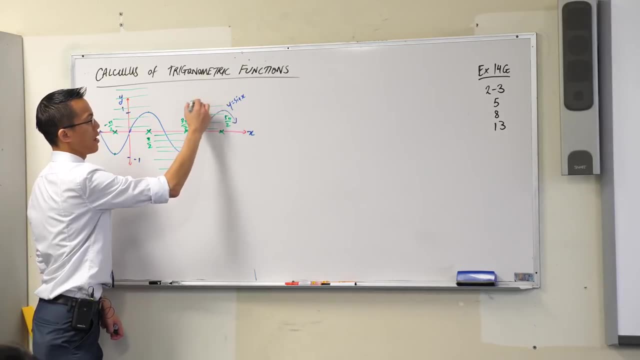 what can you tell me about the gradient there? It's decreasing And then, predictably, you get it reversing and coming back up here. Now this is interesting, right? The gradient seems to be doing the same thing over and over again. 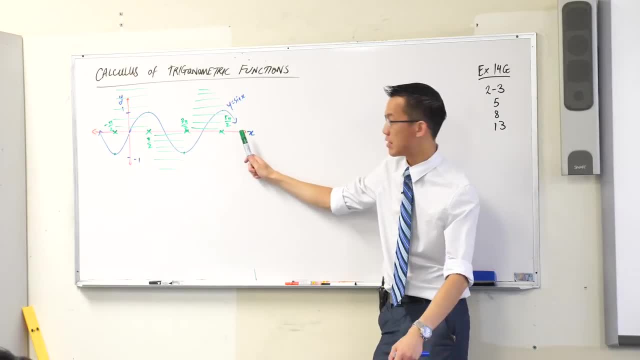 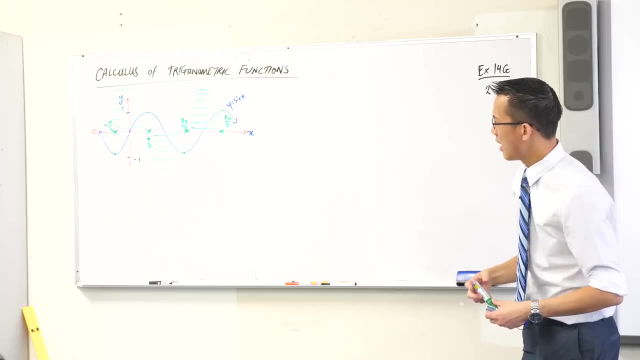 It hits 0 a whole bunch of times, repeatedly, and there's no reason why it wouldn't continue doing that. And it also seems to be doing this up and down and up and down, right. In other words, it's periodic. The gradient seems to be repeating over periods of time. 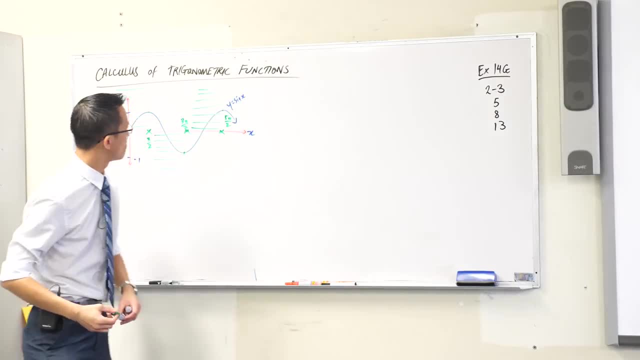 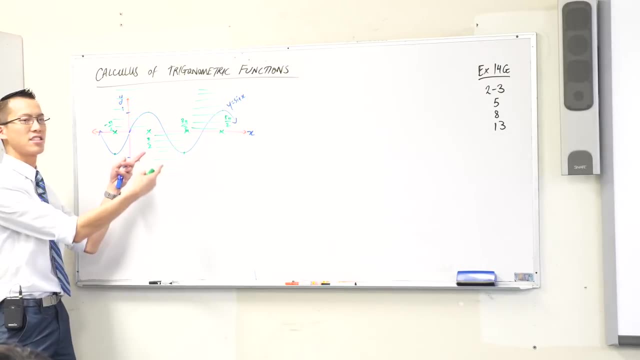 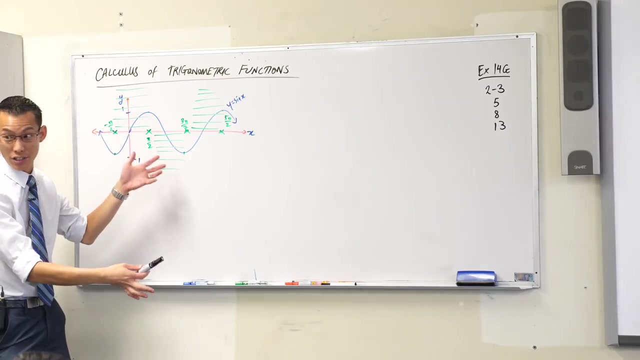 Why would the gradient be periodic? Because the function I'm thinking about right now, the sine curve, it's periodic. So therefore it stands to reason that its gradient ought to be. Now think about this for a second. The gradient function is a periodic function. 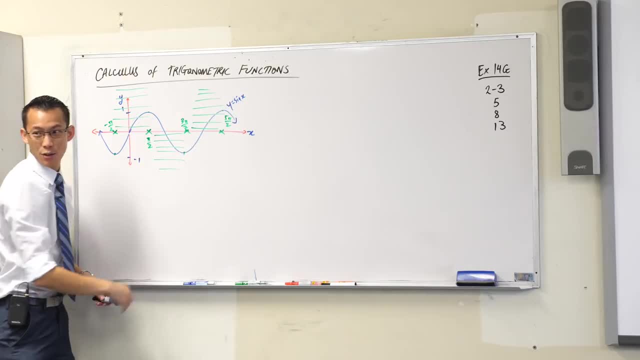 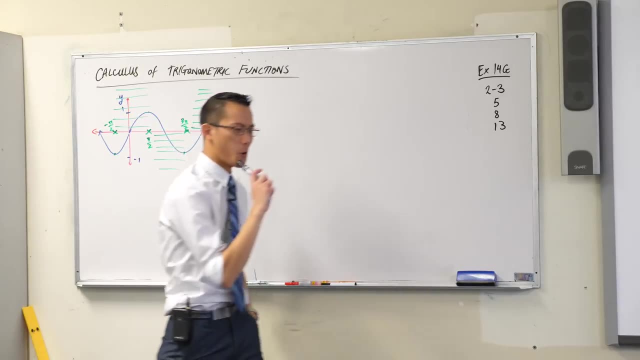 It goes up and down and up and down, and it goes through these particular x-intercepts: Pi on 2, 3, pi on 2, etc. If only I knew a function that was periodic and went up and down, and up and down. 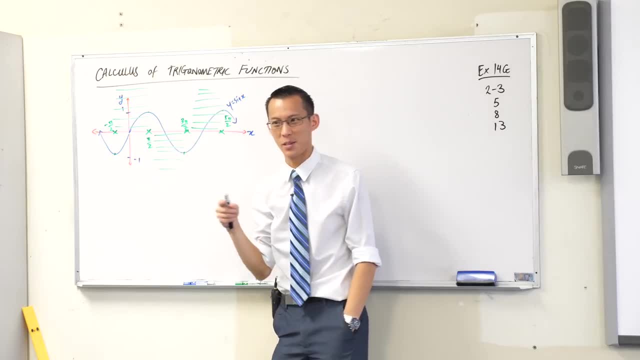 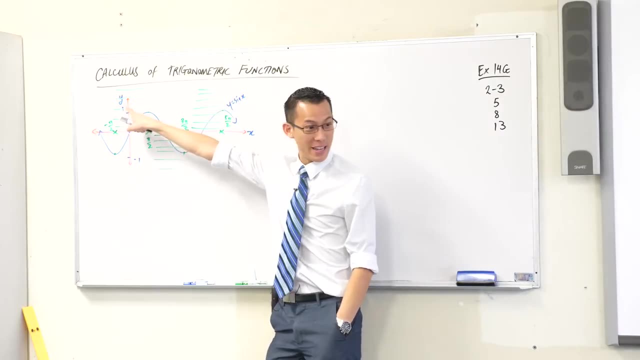 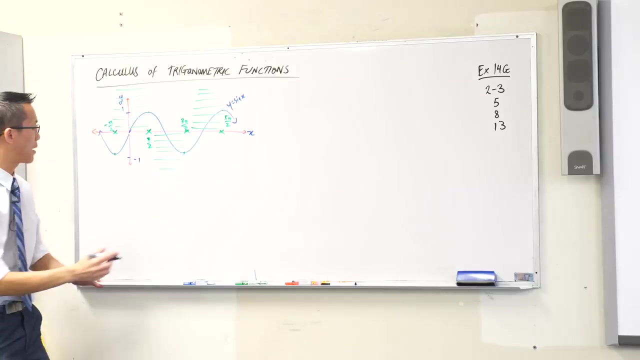 and had these particular values that it passes through. Does anyone know one that does? Have a look? It starts up here and then it goes down and then it comes up. That sounds a whole lot like cosine, right? And just have a think about this.